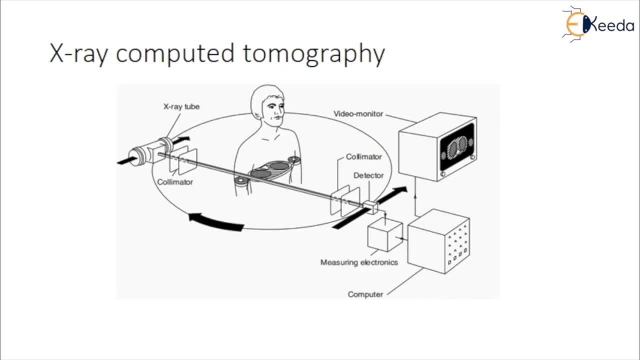 Various techniques have been applied in an effort to overcome this limitation, but the most powerful technique which has been used till now is computed tomography. The conventional tomography was developed to reduce contrast. In this arrangement, the X-ray tube and the photographic film are moved in synchronization so that one plane of the patient under examination remains in focus, while all the other planes are blurred. 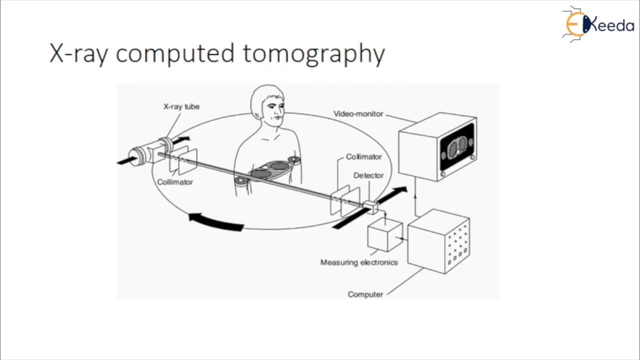 In computed tomography, the picture is made by viewing the patient via X-ray imaging from numerous angles, by mathematically reconstructing the detailed structure and displaying the reconstructions. The Greek word tomography refers to the image that was consisted of: prime, images that are not revisited in advanced modeling and Cambridge. 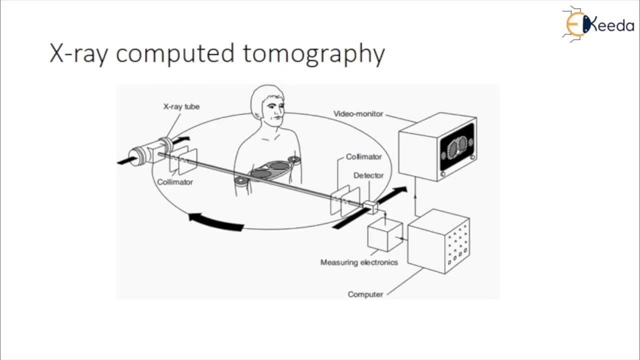 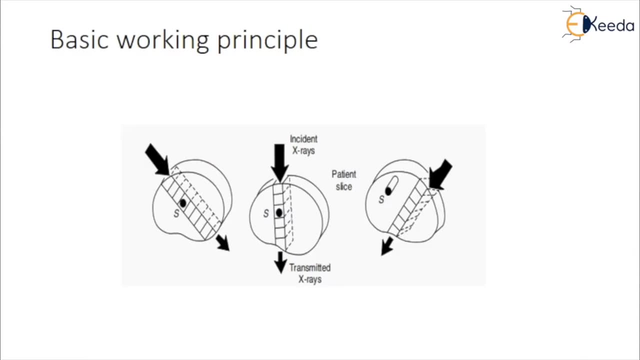 Enterprise products. It has beenабilder goodbye, Goodbye, Goodbye again, Goodbye again, Goodbye, Goodbye, Goodbye, Goodbye, Bye, Goodbye, Goodbye, Goodbye. and trans-radiates the patient from various angular projections. 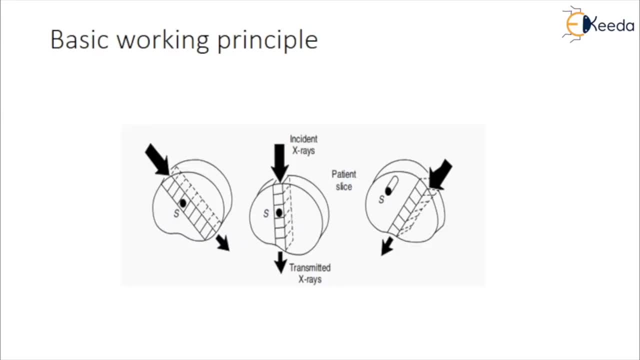 With the aid of collimators, pencil-themed beam of X-ray is produced. A detector converts the X-radiation into an electrical signal. measuring electronics then amplify the electrical signal and convert them into digital values. A computer then processes these values and computes them into a matrix line density distribution pattern. 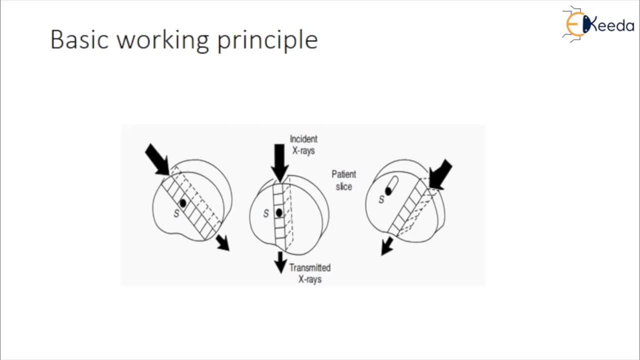 which is produced on a video monitor. as a pattern of gray shade, It is around us across the relevant sections, which is how the measurements are made. The patient lies on a motorized coach and is moved into the aperture of gantry, with the location to be accurately determined by means of narrow strip of light. 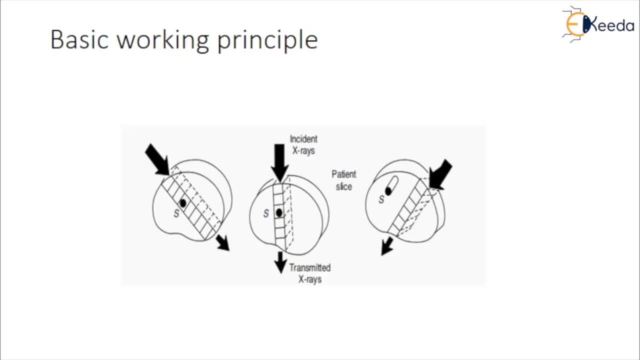 that falls on the body from the gantry and eliminates the section to be examined. From the keyboard mounted on the operating console, details such as patient's code, the name of the hospital, are fed into the system and the patient's name is displayed on the operating console. 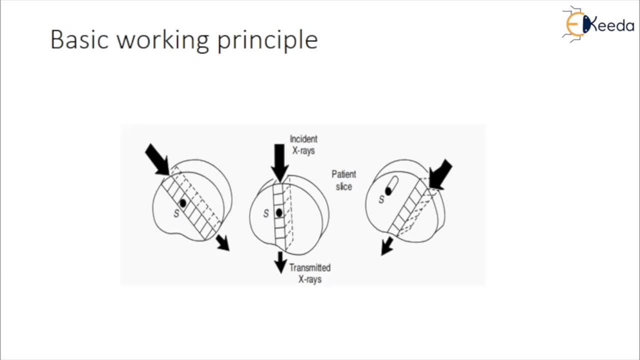 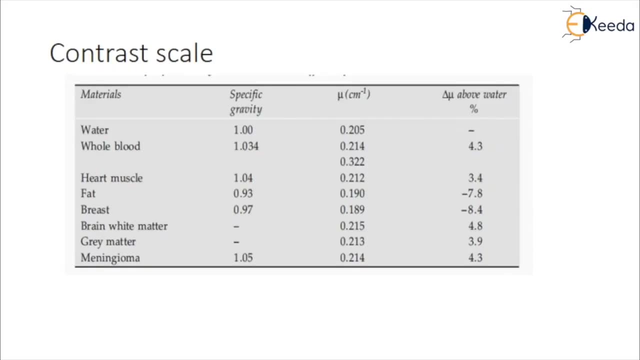 The patient's name is displayed on the operating console. and the patient's name is displayed on the operating console And the settings for X-ray parameters for the scan are made. Contrast scale: the linear attenuation coefficient of a tissue is represented by the scanner computer. 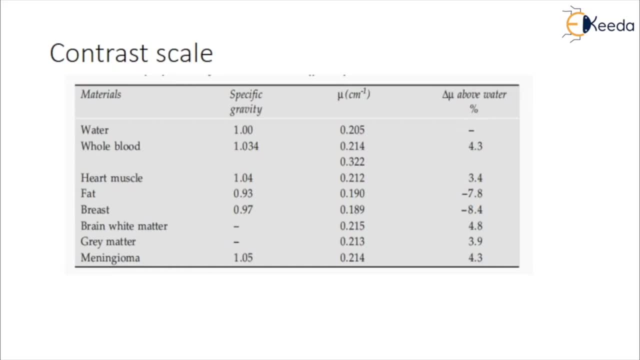 as an integer that usually range in values from minus 1000 to plus 1000.. These integers have been given the name Hans Phil. The materials used for specific gravity and attenuation coefficient for various materials is shown on the screen In this slide. water has a specific gravity of 1.0. 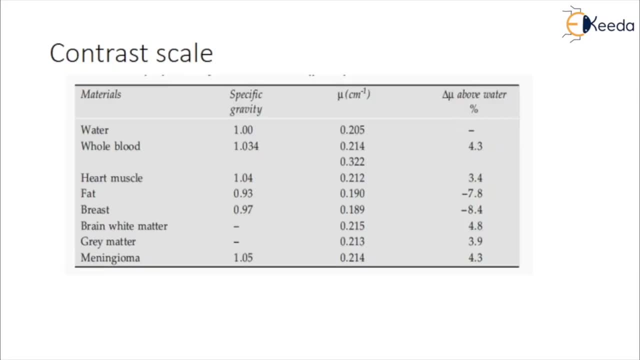 Whole blood is 1.034.. Heart muscle is 1.04.. Pat muscle is 0.93.. And attenuation coefficient is 0.190.. Breast is 0.97.. And attenuation coefficient is 0.189.. Brain water is 0.215.. 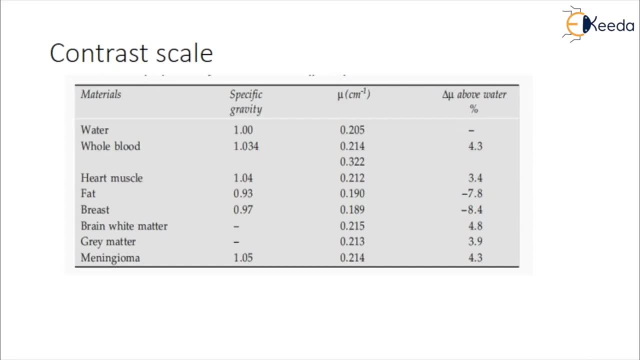 Grey water is 0.190.. Grey water is 0.190.. Grey water is 0.213.. And attenuation coefficient is 0.214.. And attenuation coefficient is 0.213.. And attenuation coefficient is 0.214. 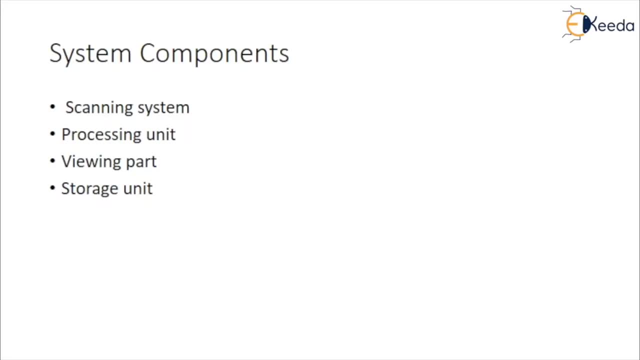 System components- Scanning system. This text plays suitable readings of the picture to be reconstructed and includes X-ray source and detectors Processing unit. This converts these readings into intelligible picture information Viewing part. It represents the information in a visual form and include other manipulative aids to assist diagnosis. 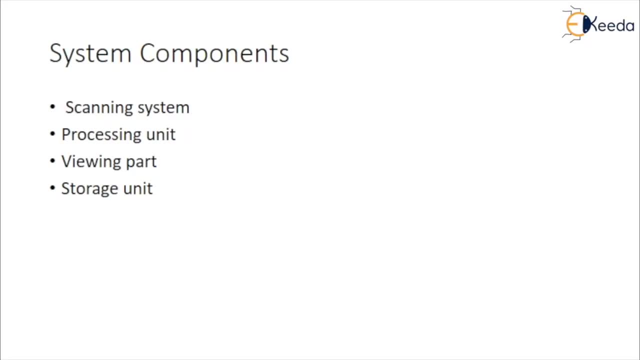 Storage unit. This enables the information to be processed. The screen is not visible. The screen is not visible. Screen vibe is stored. Screen vibe is stored for subsequent analysis. Scanning system. The purpose of the scanning system is to acquire enough information to reconstruct a picture. 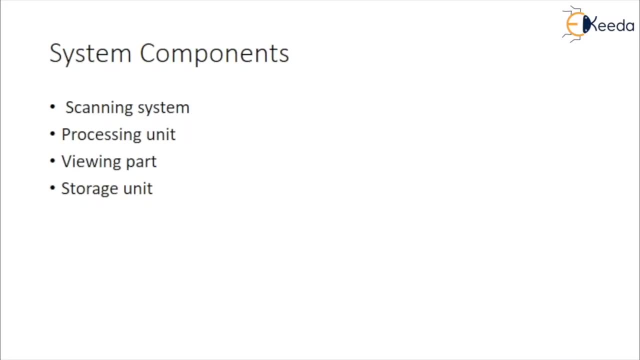 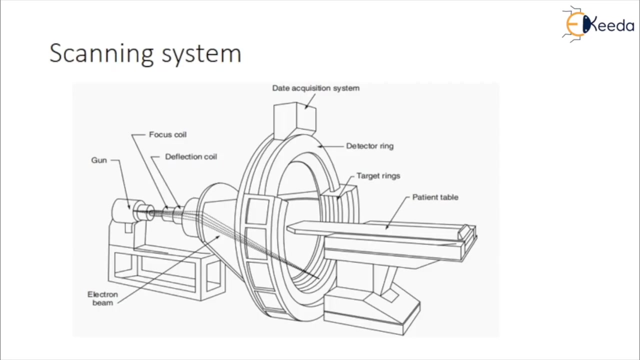 for an accurate diagnosis, A sufficient number of independent reading must be taken to allow picture reconstruction with the required spatio, resolution and density discrimination. for diagnostic purposes, The readings are taken in the form of profiles when a plane parallel X-ray beam is applied, applied on the surface of the body to passing through the required section, and profile is 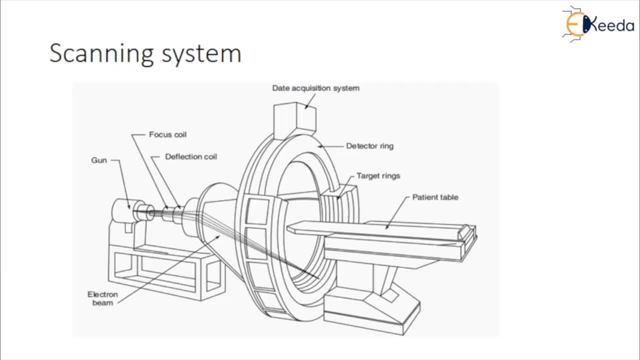 defined as a density intensity of the emergent beam plotted along the line perpendicular to the x-ray beam. These profile represent a plot of the total absorption along each parallel x-ray beams. If thus follows that the higher the number of profiles obtained, the better is the resulting. 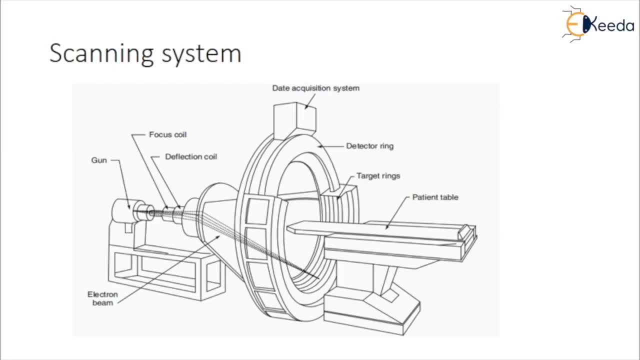 picture. Electron beam coupled tomography differs from conventional CT in terms of speed and method of generating the x-ray. The conventional CT scanning an x-ray tube and an x-ray detector are mounted across each other on a circular frame and rotate around the patient In electron beam. 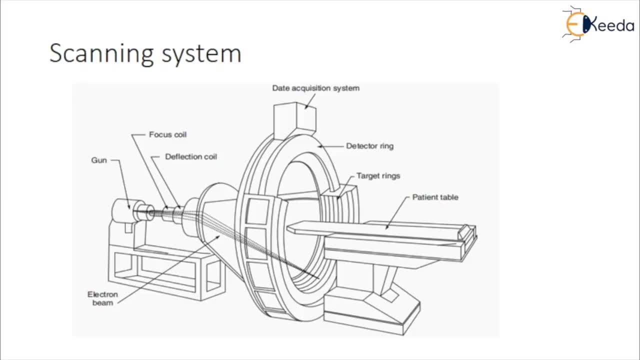 tomography. the electron beam sweeps back and forth through a magnetic field. The impact of the electron beam on a semi-circular tungsten array underneath the patient generates the x-ray beam. The x-ray beam is used to generate the x-ray beam. The electron beam is used to. 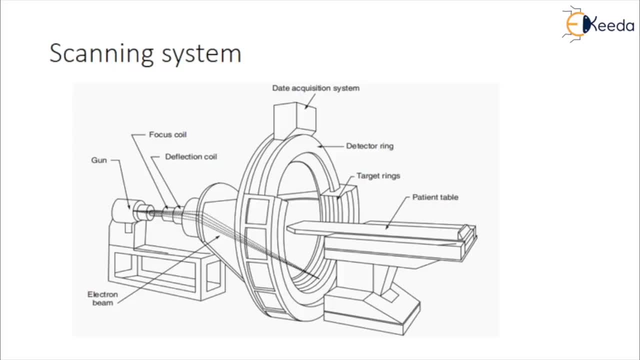 generate the x-ray beam, The electron beam on a semi-circular tungsten array underneath the patient generates the x-ray beam, and the x-ray detectors are mounted on a semi-circular array above the patient Because an x-ray tube and x-ray detector are heavy moving parts weighing up to 250 kg. it. 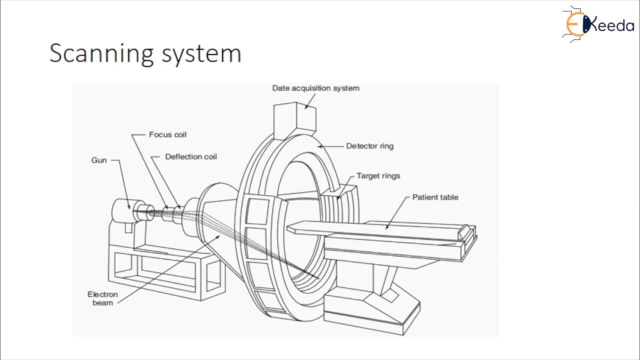 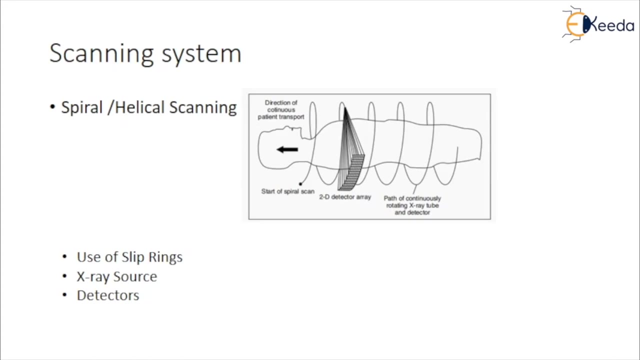 takes one second or more to take all the snapshots which are later reconstructed to form an image of one slice of a body with a conventional CT scanner. Spiral and helical scanning: This is a scanning technique in which x-ray tube rotates continuously around the patient. 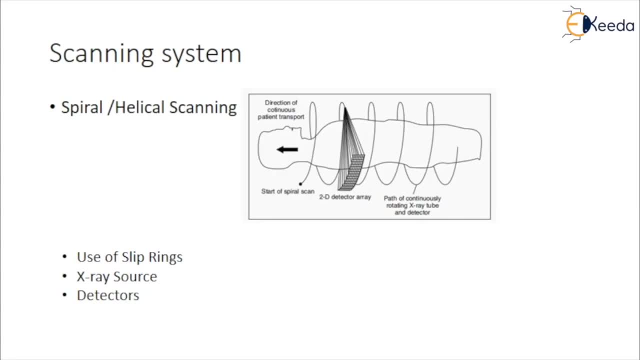 while the patient is continuously translated through the fan beam, The focal spot, through traces, a helix around the patient, The projection data is obtained, allowing reconstruction of multiple contiguous images. This technique has been developed for acquiring images with faster scan times and to obtain fast multiple scans for three-dimensional imaging to obtain and evaluate. 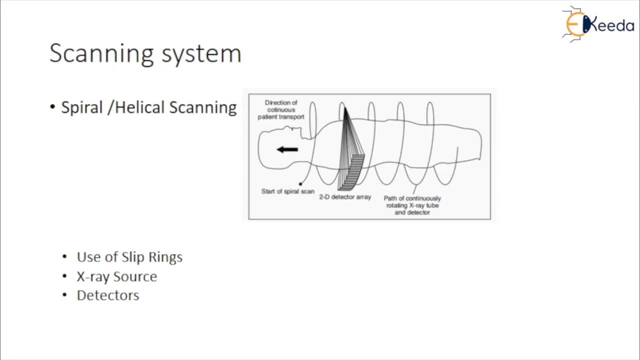 the volume at different locations. Multiple images are used to scan multiple images at different distances. The patient is moved through the gantry in a smooth, continuous motion rather than stopping for each image. The reconstruction algorithms are more complex because they need to account for the spiral or helical path traversed by the x-ray source. 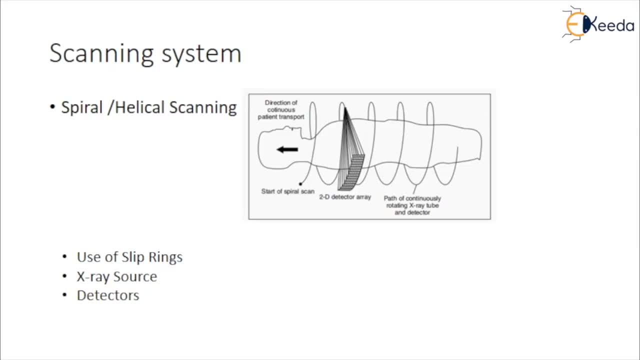 around the patient. Use of slip rings. In a conventional CT scanner, the input power is applied to the transformer, which is located separately from the gantry. The transformer is located separately from the gantry. The transformer is located separately from the gantry. The transformer steps up the voltage to the level of 80 to 150 kV. The high voltage 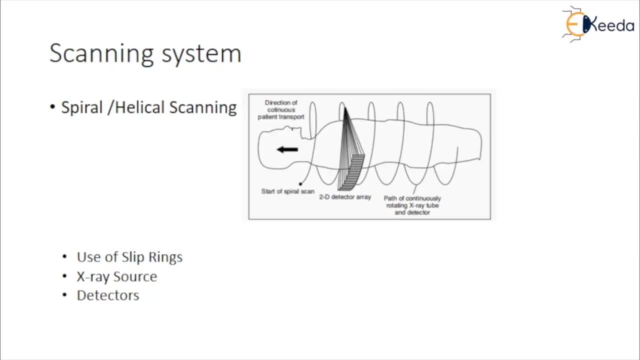 is applied by a special cable which are attached to the x-ray tube in the gantry. A sophisticated cable management system allows the tube free across axis for about 400 degrees of rotation in either direction. Therefore, the tube must be rotated first in one and then in the opposite.